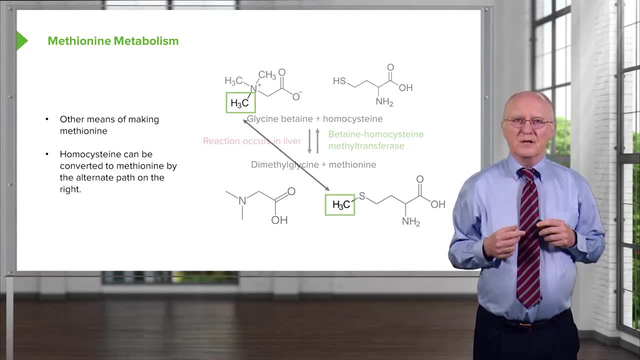 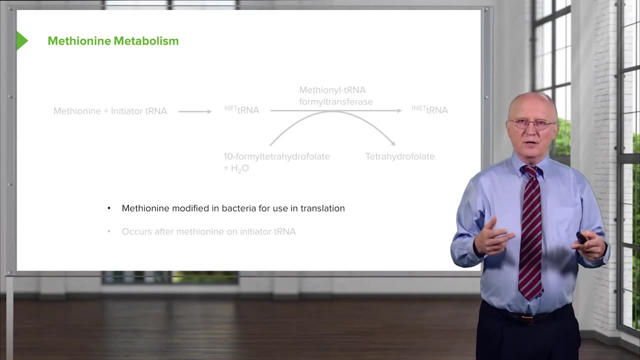 And the reaction here occurs in the liver. We see the transfer of the methyl group, as occurs right here Now. methionine is modified in bacteria before it is put into making proteins. We remember in bacterial translation that the very first amino acid that makes it into 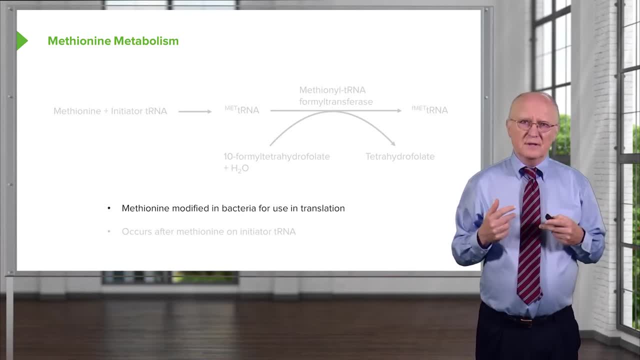 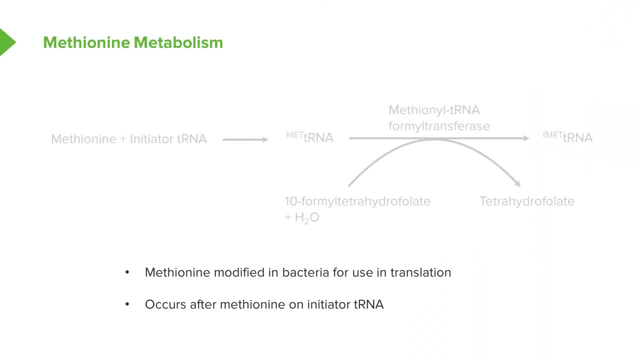 proteins is not methionine, but a modified form of it, And that's known as formylmethionine. And that's known as formylmethionine. So this set of reactions I'm going to show you shows how that formylmethionine is made. 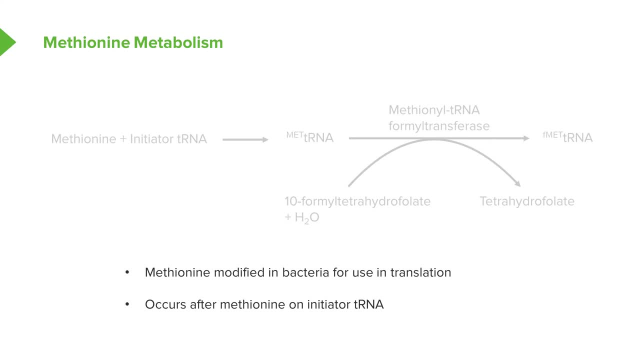 Like the synthesis of selenocysteine, formylmethionine is made by modifying in a methionine, that's on a transfer RNA. This is shown in this set of reactions. Methionine combines first with its initiator, tRNA that's used to put it into the proteins. 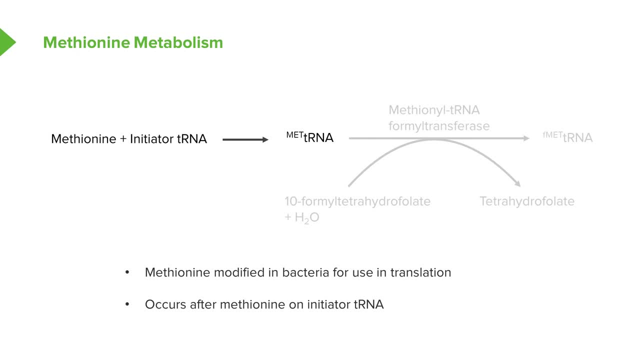 during the process of translation. This produces the methionine joint to the tRNA And in the reaction we see that methionine is made by modifying methionine, that's, on a transfer RNA. This is shown in this set of reactions. 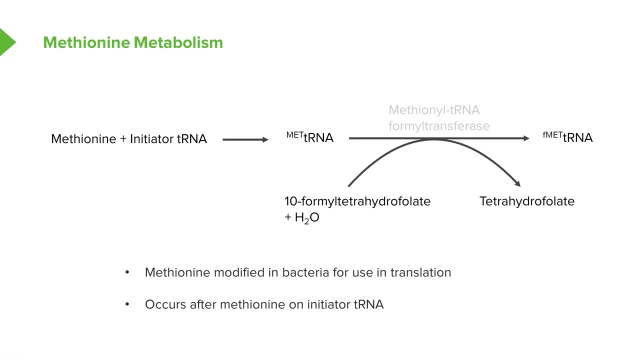 And in the reaction that makes formylmethionine we see that the formyl group actually comes from 10-formyl tetrahydrofolate and produces the formulated methionine on the transfer RNA. The product of that reaction makes tetrahydrofolate and the enzyme catalyzing it is methionine. 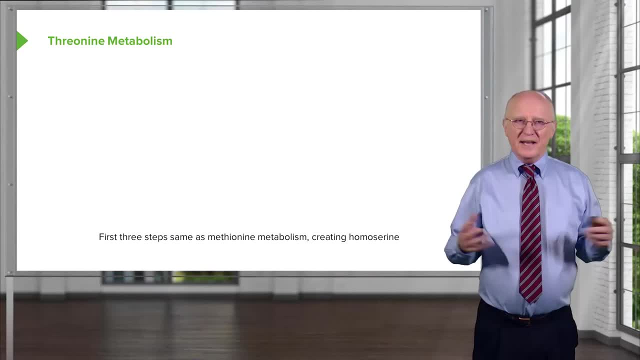 tRNA formyl transferase. The next amino acid metabolism we will consider is that of threonine. Threonine's metabolism overlaps a bit with methionine metabolism. The first three steps of the synthesis of threonine from aspartate are the same as the. 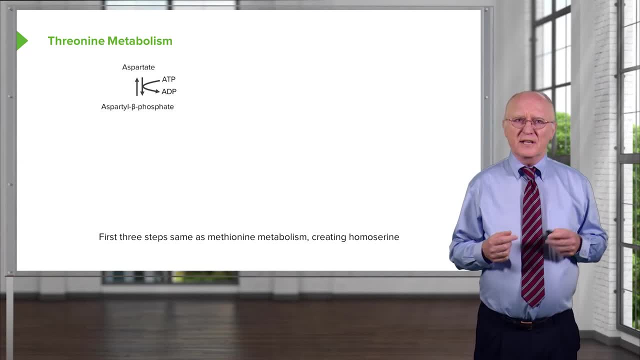 first three steps in the synthesis of methionine: Threonine is converted to beta-aspartate semi-aldehyde by a reduction, and the homoserine is created from the last intermediate by a reduction as well. These three steps also happen in the synthesis of methionine. 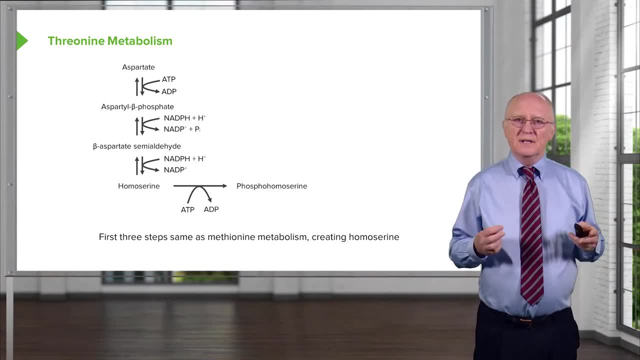 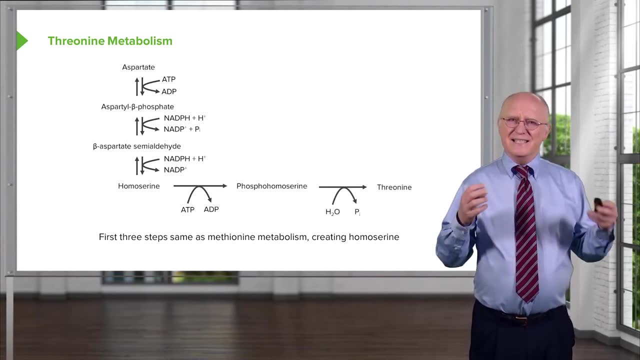 In the next step of the process, homoserine is phosphorylated to make phosphohomoserine using energy from ATP, And then phosphohomoserine is dephosphorylated, and that dephosphorylation involves a molecular rearrangement.